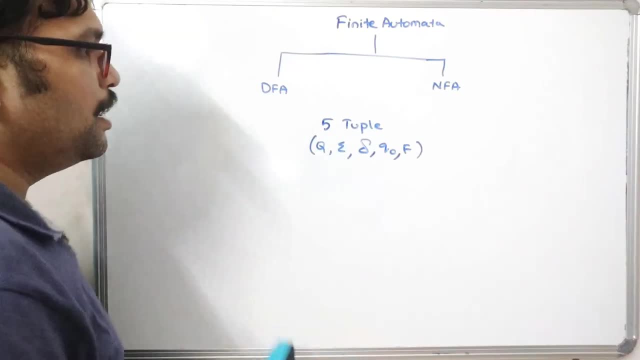 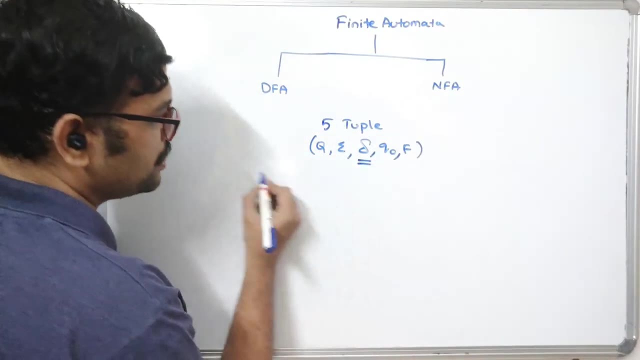 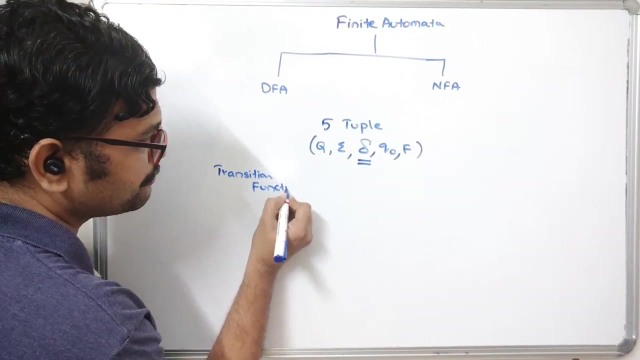 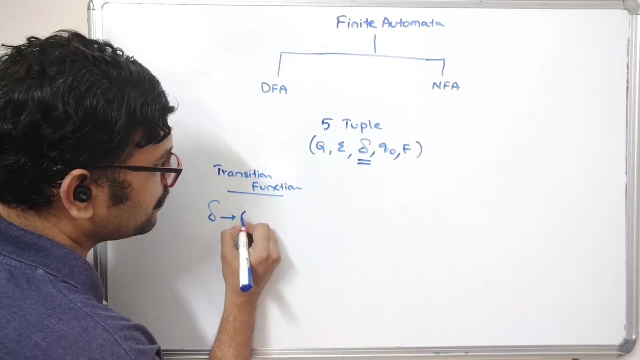 That means one initial state and multiple final states. Now we will see. the difference between DFA and NFA is only On the transition functions. So here the transition function. Let me explain about this one. Here the transition function can be represented as: So, though, can be represented as Q cross. 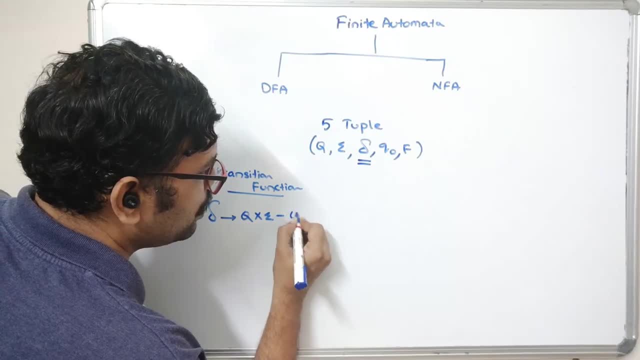 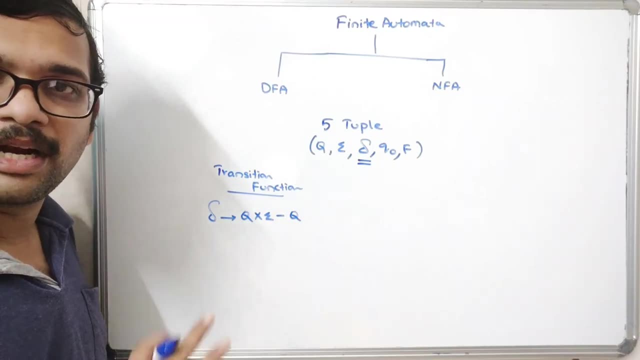 product sigma will give. The result will be in Q itself. Okay, So Q is nothing but number of states. Q is nothing but number of states. So I will explain. Let me explain about this one by taking one example And coming to the NFA. here, the transition. 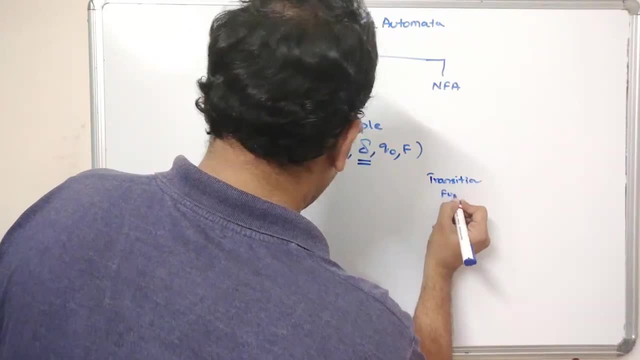 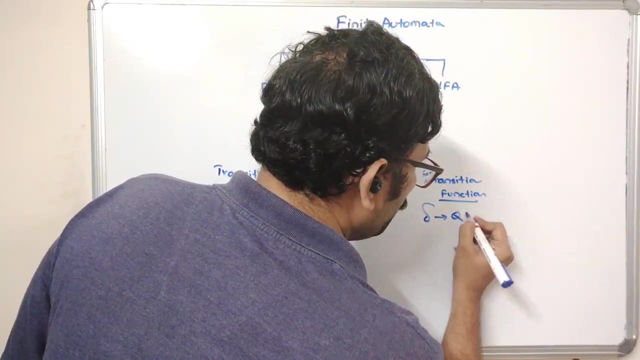 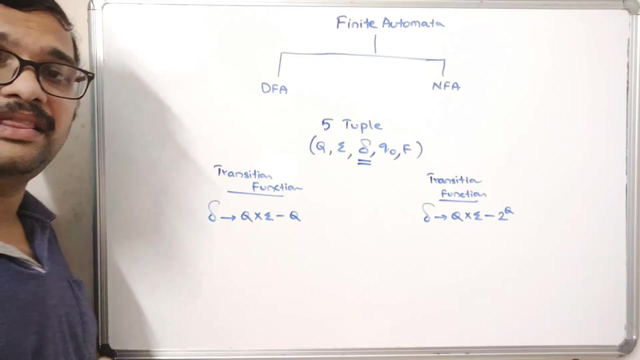 function. Here the transition function can be written as: So: transition function. So the same thing. Q cross product. the sigma will be given at two power Q. That means it can be anything. power set of Q- Okay, This is nothing but power set of Q, Okay, So this: 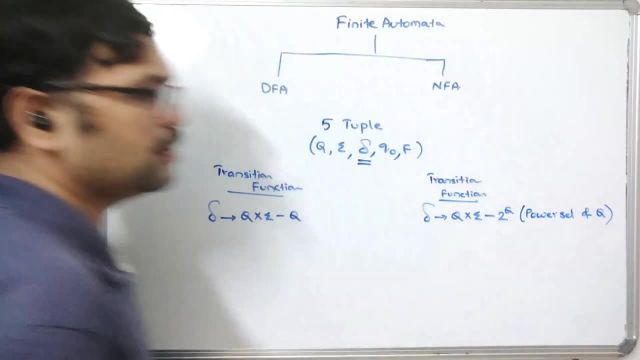 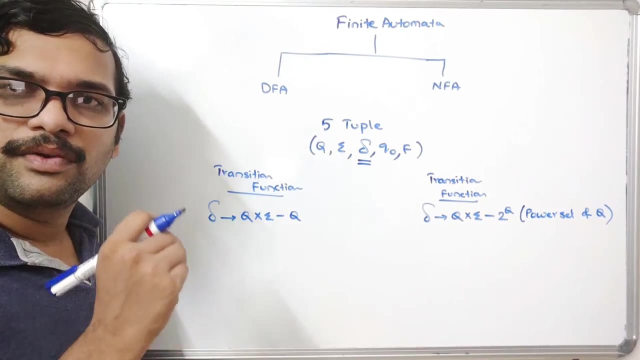 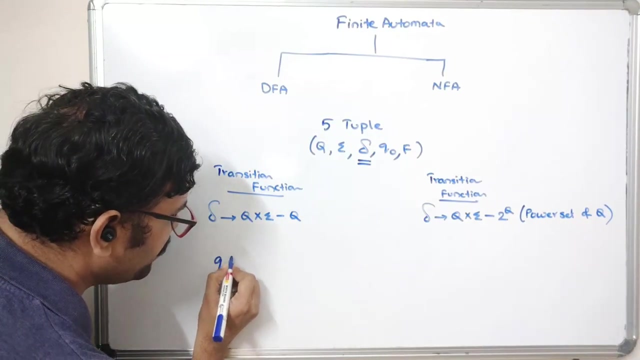 is nothing but power set of Q. So let me elaborate this one. So, for example, here, for every state with one input symbol, there should be a transition. Okay, So for example, let us take two states in a simple example: Q naught, So this is a starting state and moves with a one. it goes. 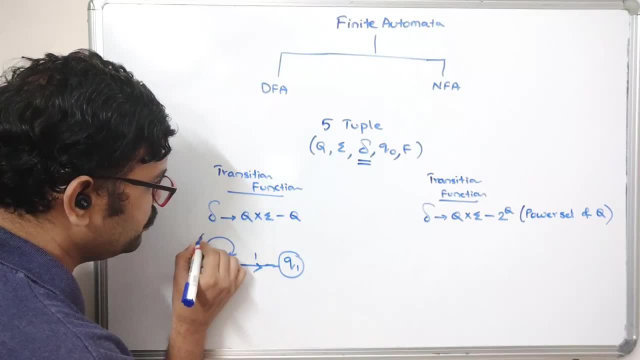 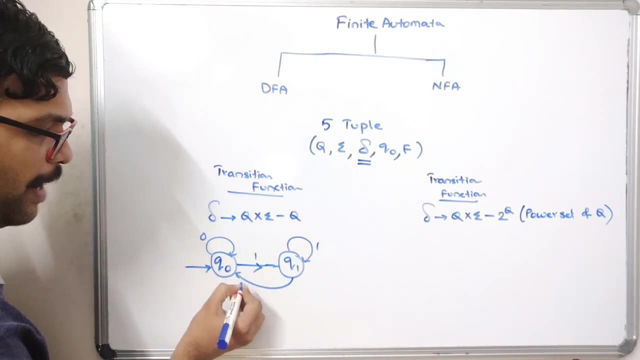 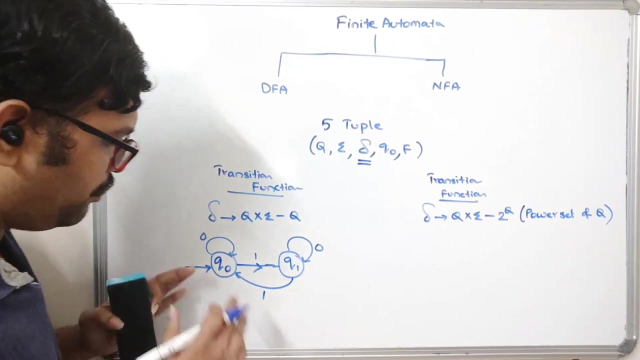 to the Q one and just give the self loop if it is zero, and give the self loop if it is one, Okay, And give the go back to here. So let us take this zero and this is one Okay. So just take this as an example. Here you can observe, if you consider, here we are having 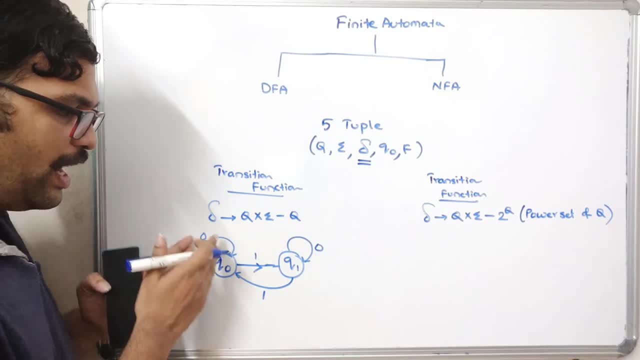 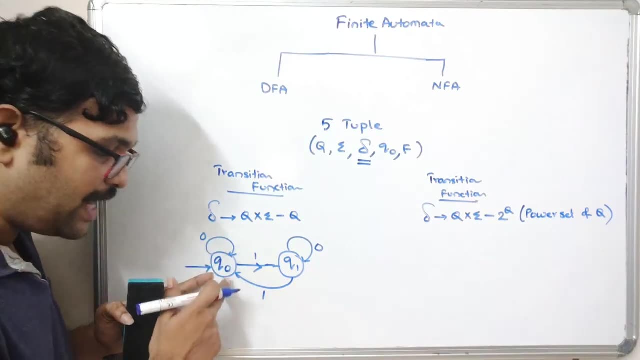 a two states. Here we are having the two states And we are having a two input symbols: zero and one. So here you can observe, Q naught. Q naught is the state which is having a transition for both the symbols zero and one. Similarly, Q one, if Q one is a state and Q one is a state. 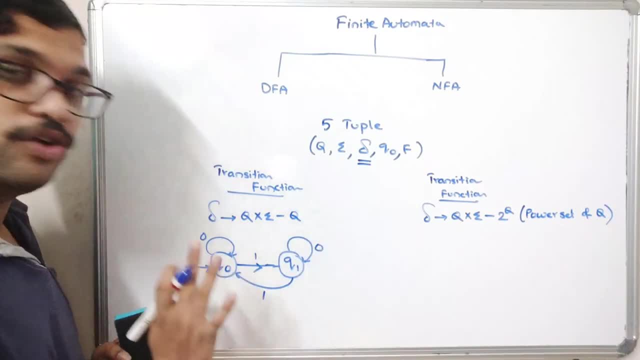 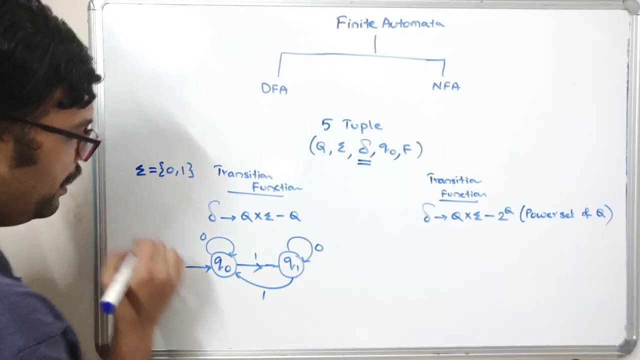 so Q one is also having the transition for both the symbols zero and one. So here let us take the sigma is equal to zero comma one. that means the two input symbols, And here you can see the Q naught on zero, Q naught on one. Similarly Q one on zero, Q one on 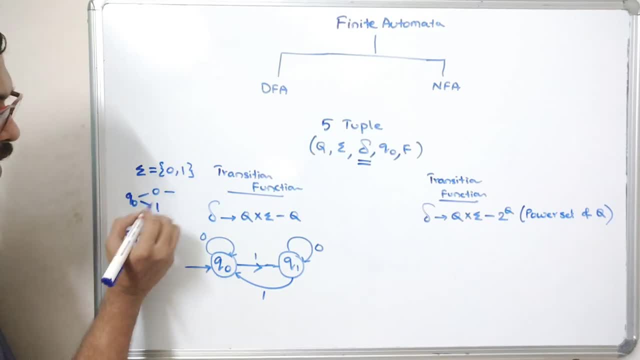 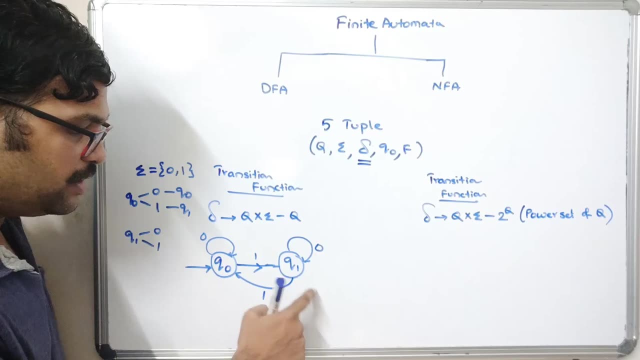 one. So here, if it is Q naught on zero, it will remain in the same state: Q one, Q naught on one, it will move with a Q one, Q one on zero And if you consider this one, Q one on zero, C one on zero and Q one as one. So let us see. 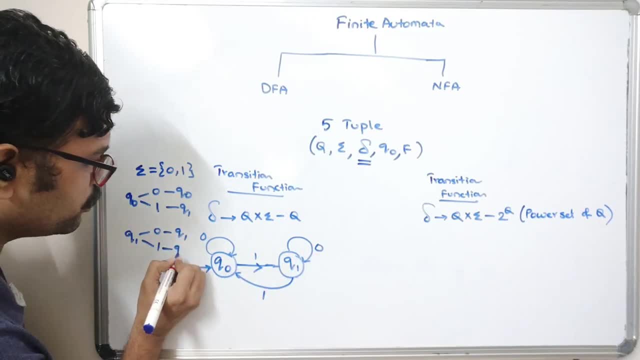 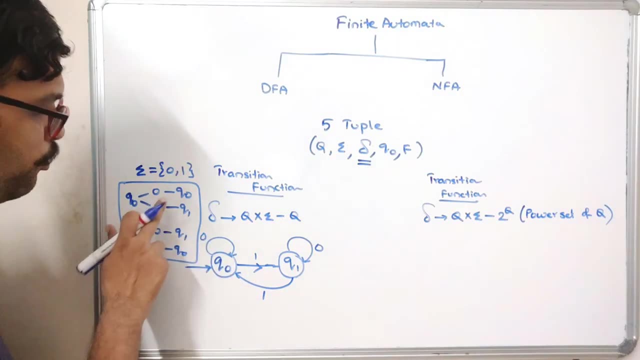 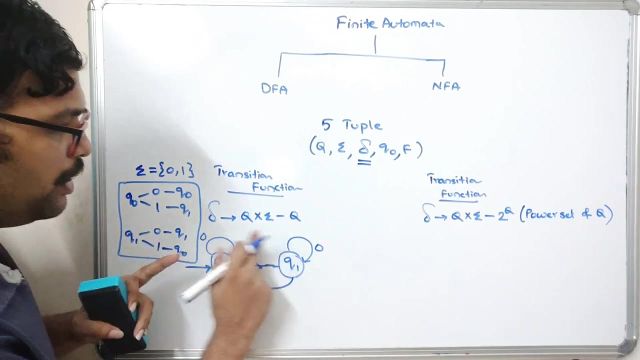 it remains in the same state. q1 on 1, it goes to the q0. so you can observe here clearly: for every transition of the state with the input symbol, there will be only one state. so there is there is a only one path. there will be only one path. so that's why we call here so 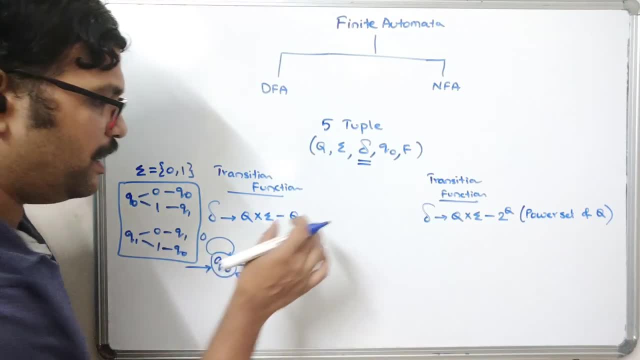 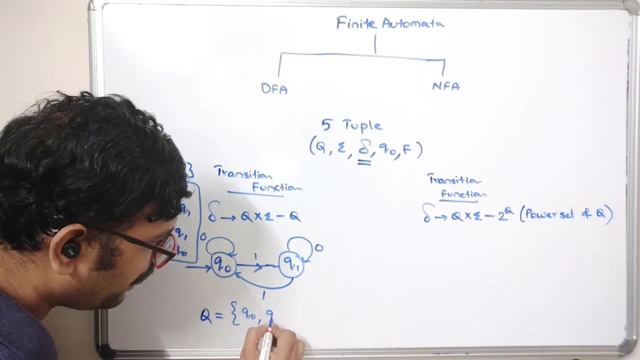 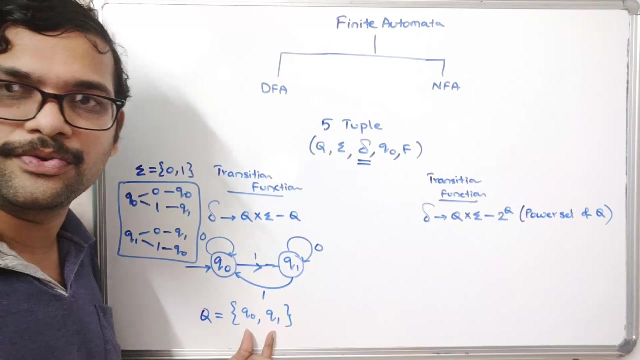 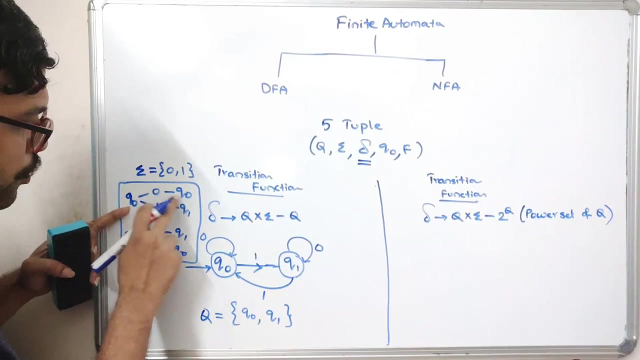 q into sigma is equal to q. q means the result will be in the set of q. so in this example you can see q is equal to q0 and a q1. so automatically for every input symbol the state can be one among this set, q set. see you can observe here q0 on 0, q0. so that is in this set. q0 on 1, q1: it is in set. 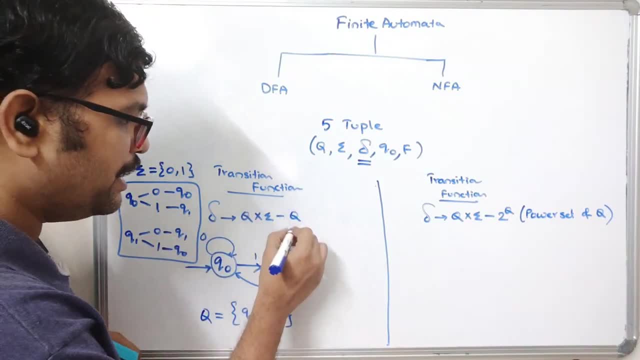 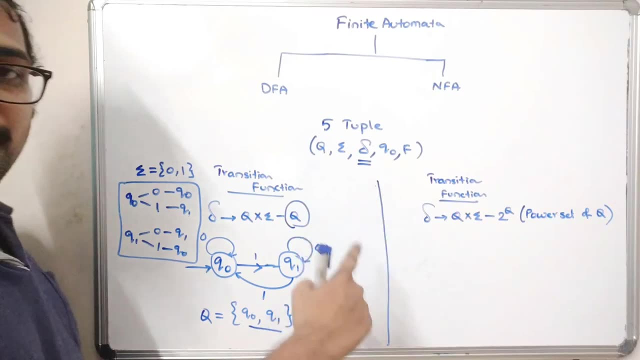 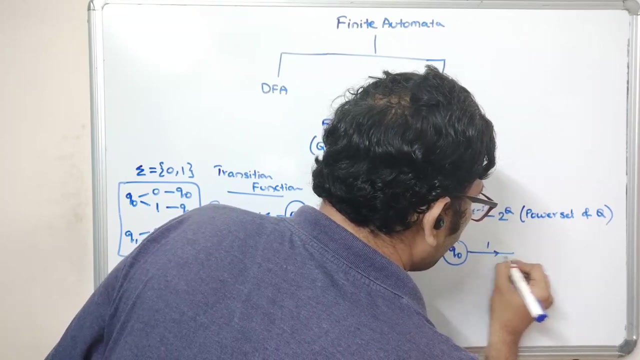 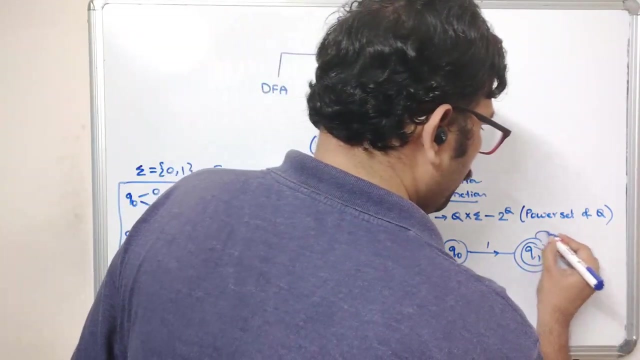 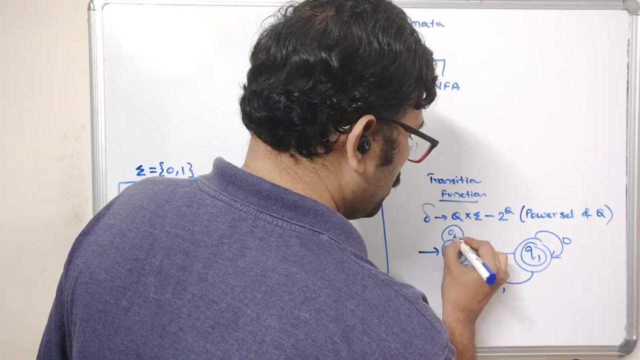 in this set, so the resultant state will be in this particular set of states. okay, one among this set of states. so so, And coming to here, that is completely different. Let us take the same example here. So Q naught, and so let us take this one. So here let us take this one as a final state and go with here 0, and here you can go with a 1 and go with a 0 comma 1.. 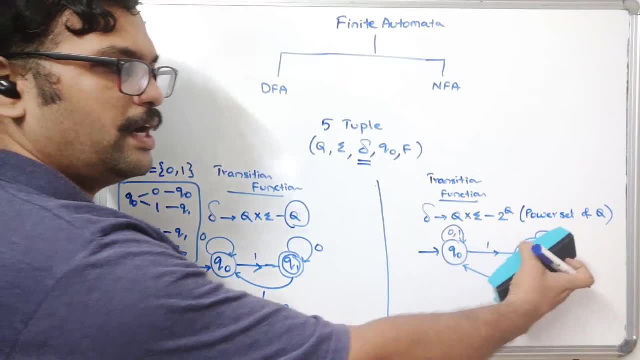 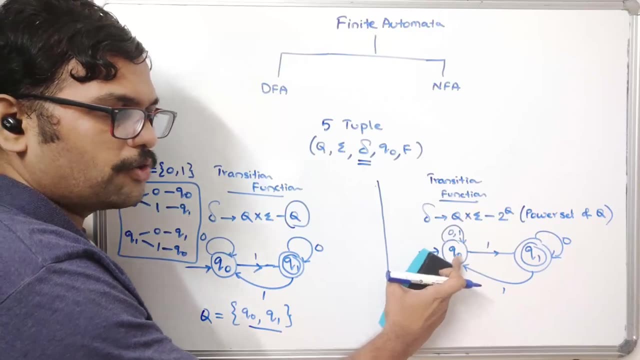 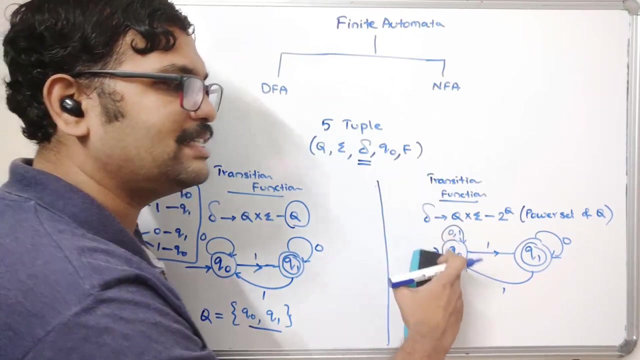 Let us take this one, 0 comma 1, and here 0.. So that means in this case. so the question: here you can see the Q naught with the input symbol 1. there are two different states, So it can remain in the same state or it can go to the Q1.. 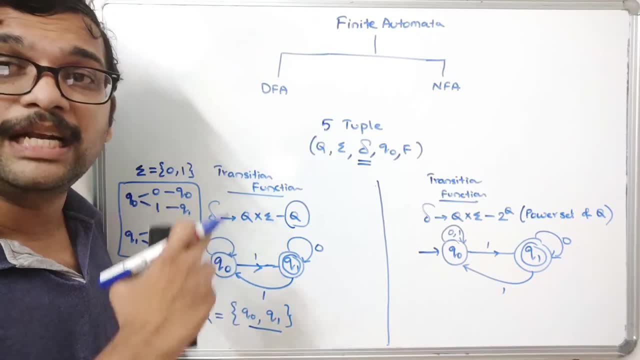 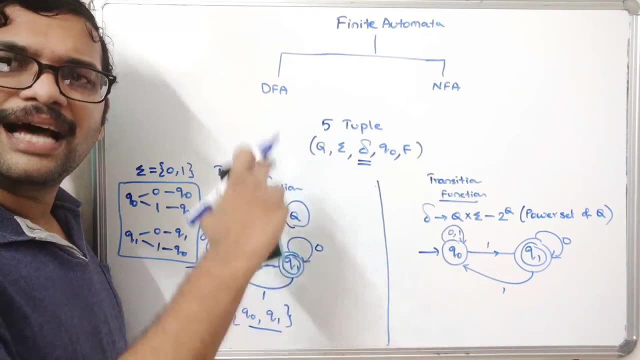 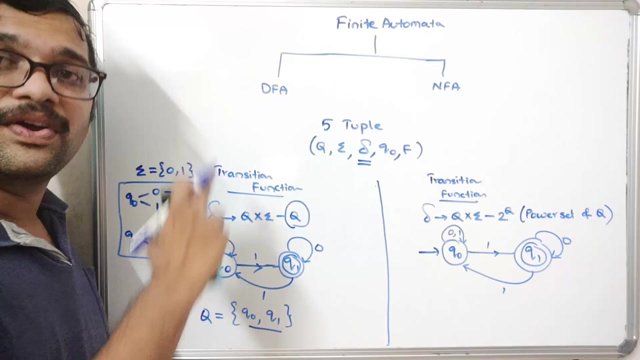 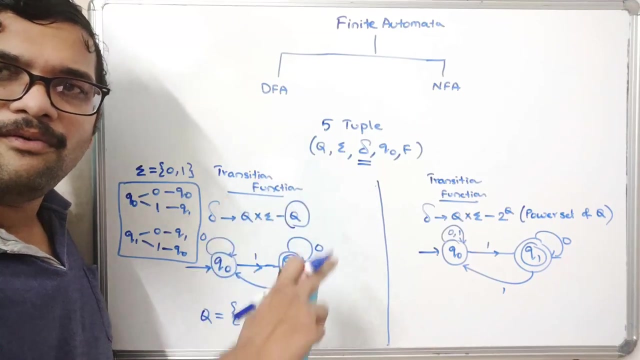 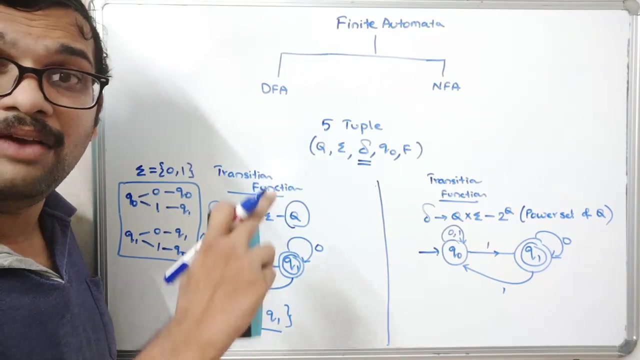 That means having a different paths, that means a multiple paths. Okay, there can be a multiple paths and if necessary, it will change its state. Otherwise we need to change it. So you need not mention the transition also. But here, not like that, For every state there should be a transition for every input symbol. So here you can see: Okay, but here it is not required to have a complete state. I mean a transition for every input symbol, A transition for every input symbol. So if it is not required, you need not go with this one. 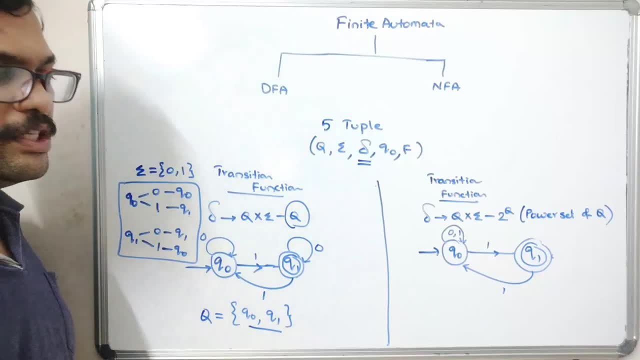 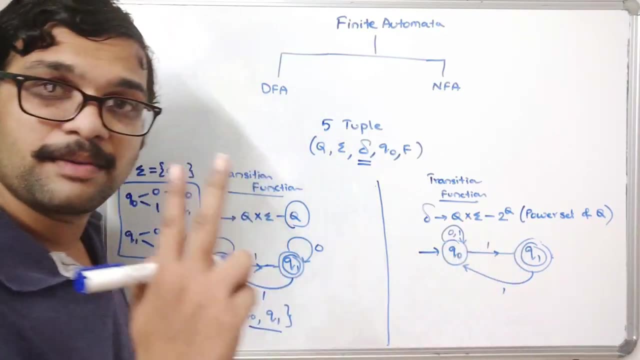 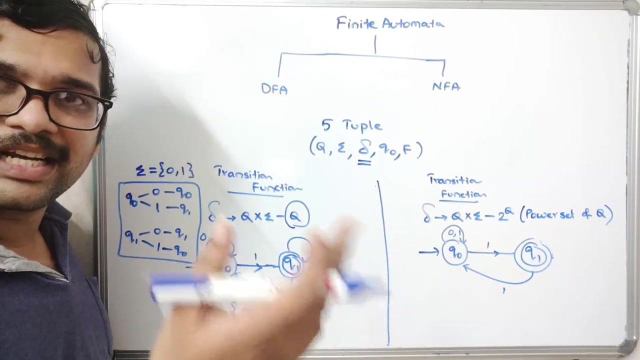 So if it is not required, you need not go with this one. So you can observe here, This is also an NFA. This is NFA because, so you can see, for Q naught two points. Just remember the two points. So one thing: So one state can change to multiple states for any one input symbol. So there will be multiple paths. That is our first point. 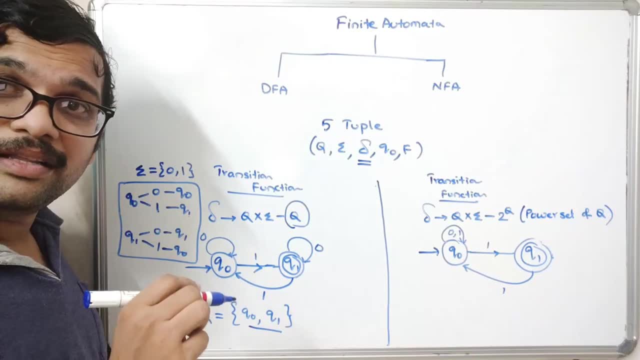 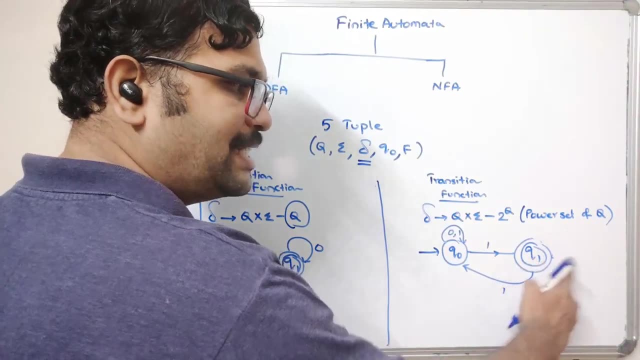 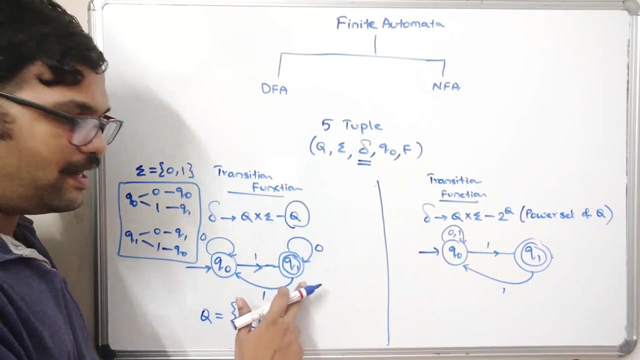 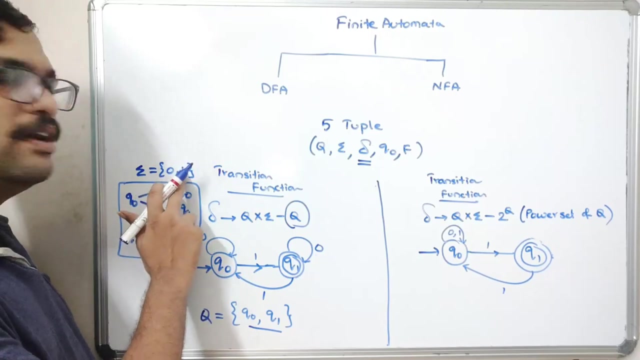 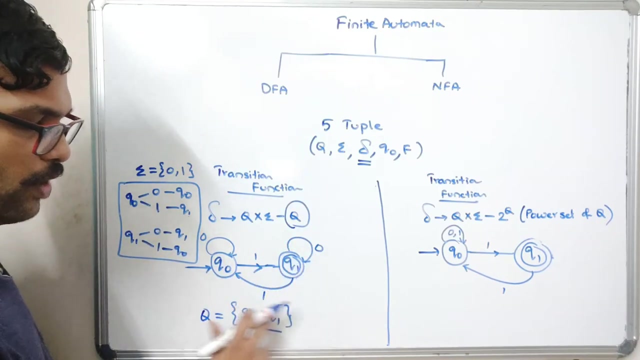 The second point: for every state there need not be a transition for every symbol. Okay, here you can see the Q1 on 0: there is no transition because it is not required here. So this is called NFA, But here it is not like that. For every state there should be a transition for every input symbol. So there are two symbols, 0 and 1.. For every state there should be a transition for 0 and 1.. So that is why Q naught with 1: there is a transition. Q naught on 0: there is a transition. Q1 on 0: there is a transition. Q1 on 1: there is a transition. 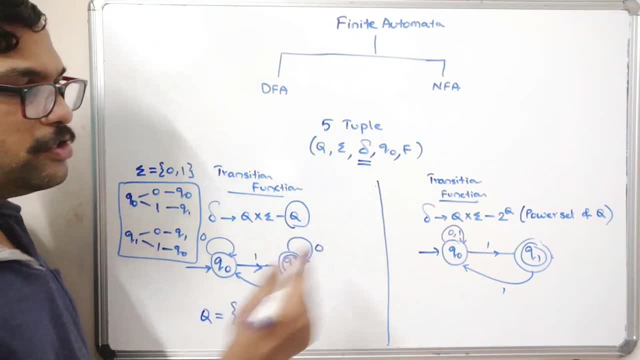 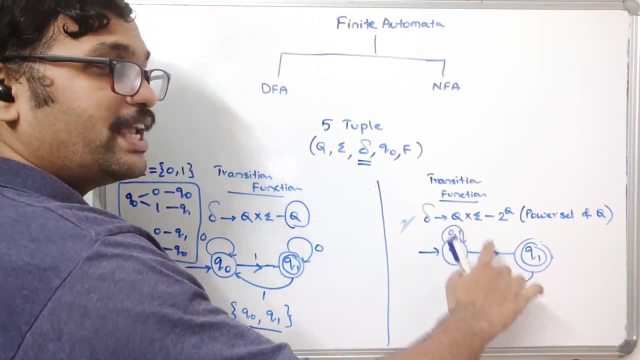 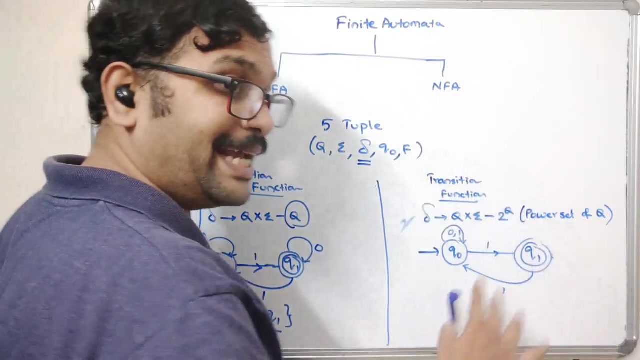 So this is the major difference between these two things. So, coming to this transition functions, you can see. So if you cross product the symbols with the states, So if you get the state, the next state, from this power set of Q, From the power set of Q, The next state can be the power set of Q. 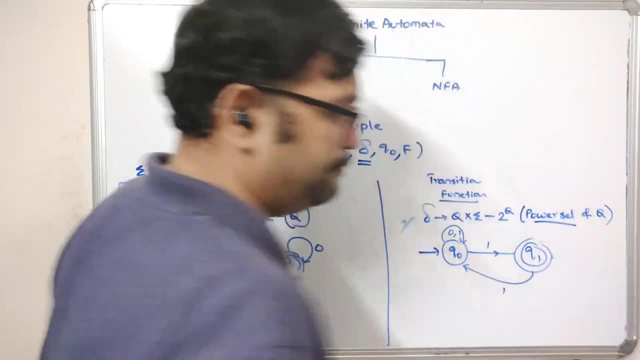 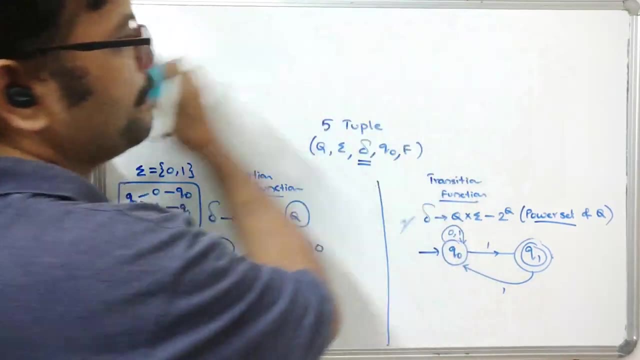 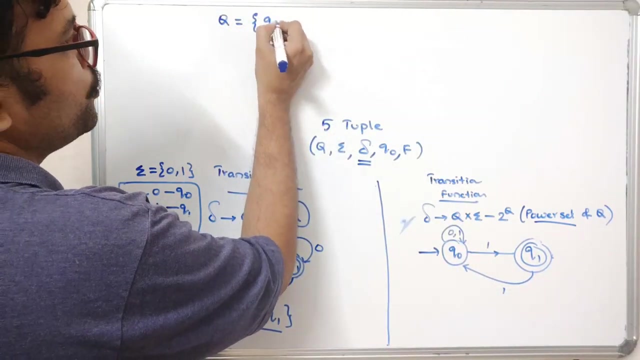 Now we will see. what is this power set, What is meant by this power set? See, for example. So I will use this one For example. So Q is having two states, So Q naught and Q1.. 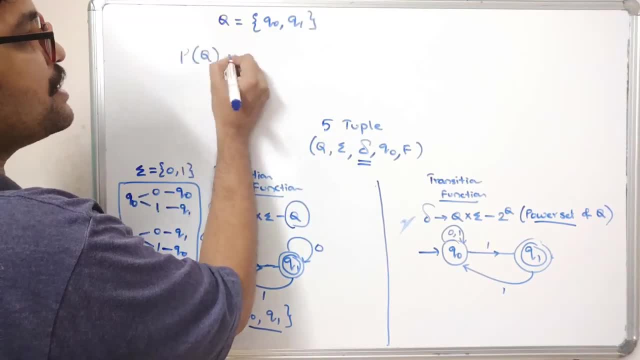 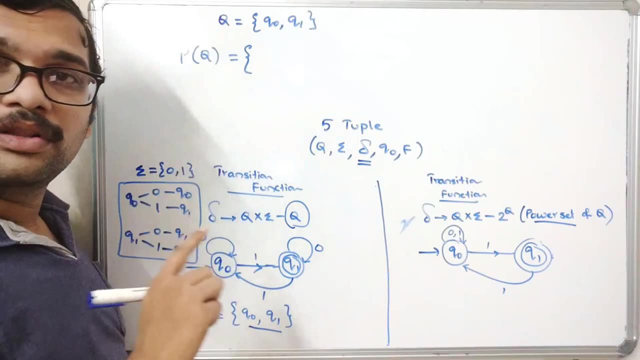 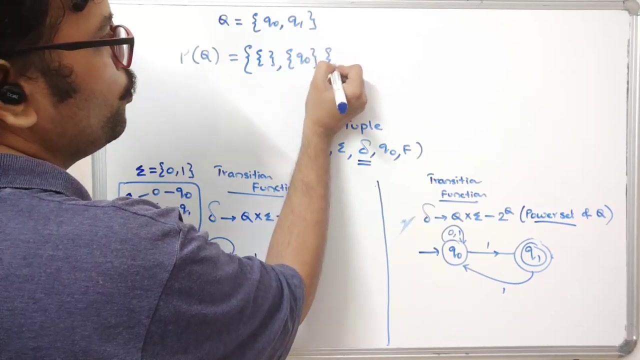 So Q naught and Q1.. Now a power set of Q. Power set of Q will be the combination of all the states, So it will include the empty set also. So one empty set will be there And Q naught is one state, Q1 is another state And Q naught, Q1 is one more state. 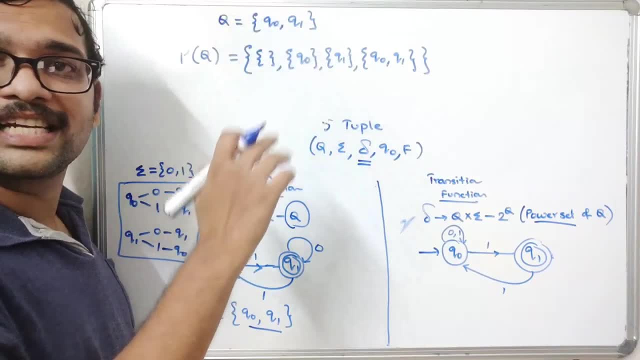 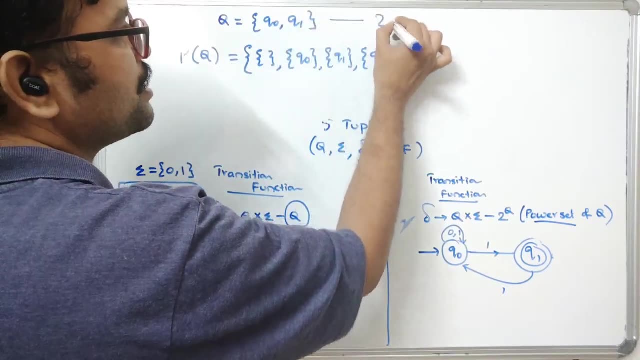 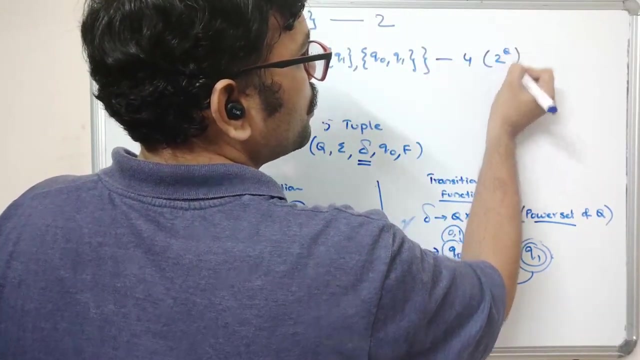 Right, So the combination of all the states. we call it as a power set. Okay, So you can see how many states are there. Two states are there. How many states are there in this power set? We are having some four. That implies two power Q. 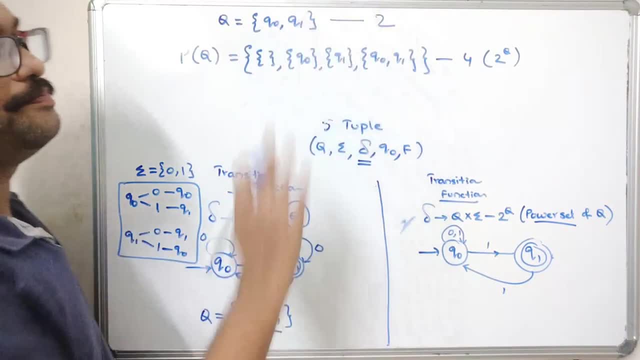 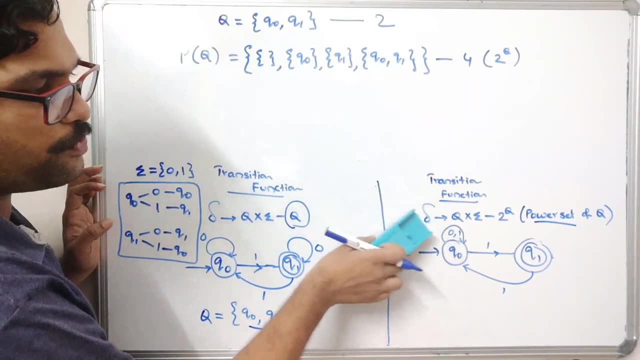 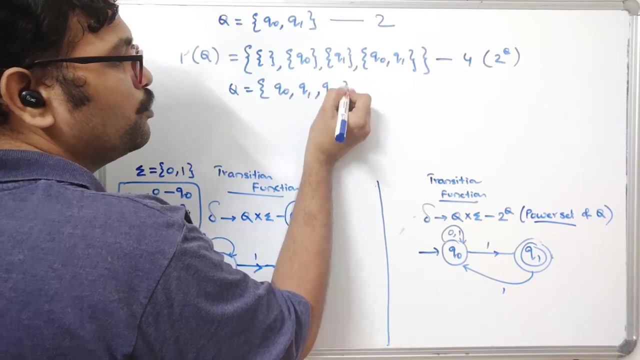 Okay, Two power Q. So if you are having three states, So I will tell you. I put the example. One more example, So I will justify this transition function. So if Q is having three, Q naught Q1 and Q2.. Three states: 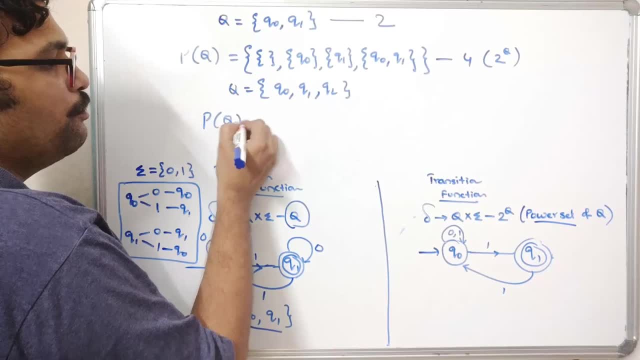 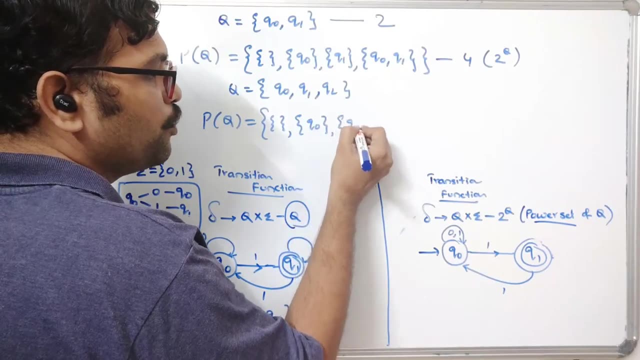 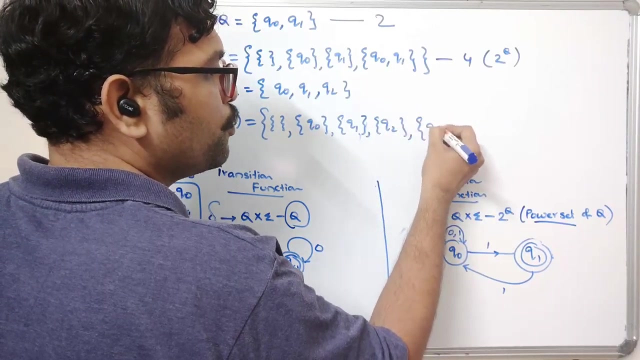 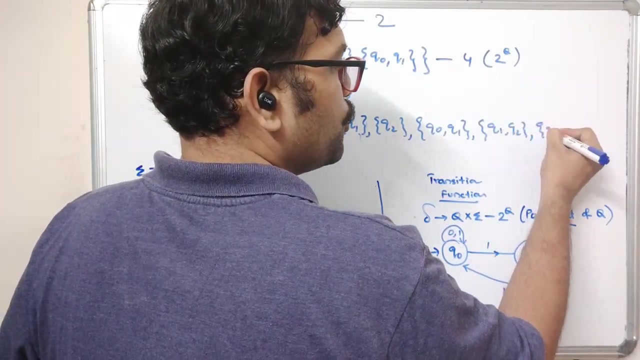 Now the power set of Q will be the combination. The first one will be the empty set, Second one the individual states. So Q naught, Q1, Q2 and combination. Q naught and Q1 is a one state, Q1, Q2 is another state, Q2, Q naught is another state. 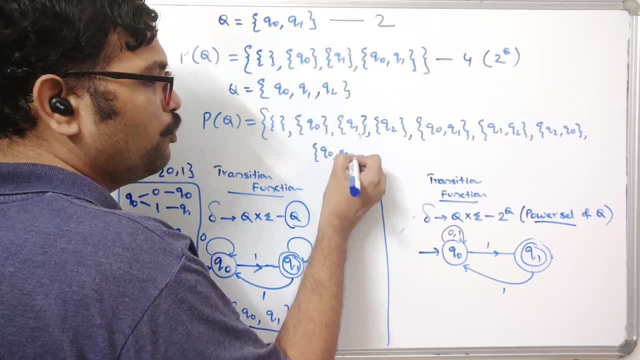 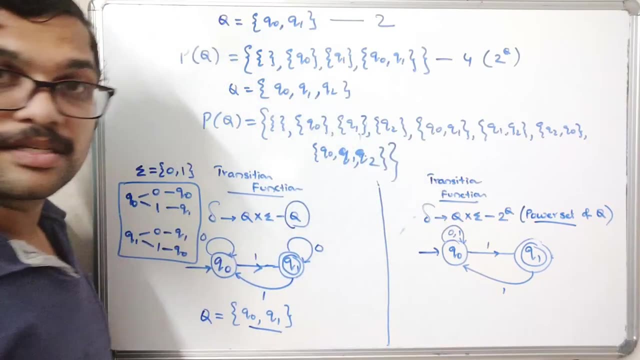 And also you can have Q naught and Q1.. Q naught, Q1 and Q2.. Right, So these are the combinations. You can count it: One, two, three, four, five, six, seven and eight. 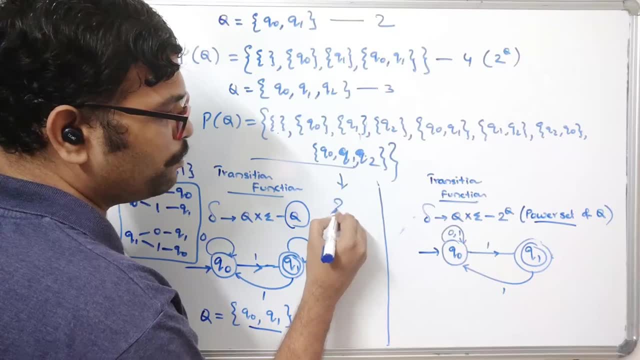 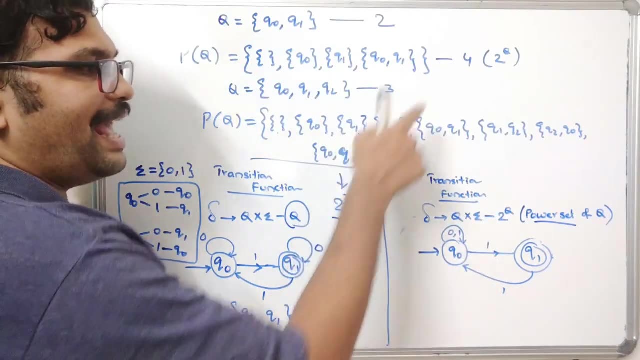 So here there are three. The power set is having two power three, Two power three Right. So that is the justification. So if in this NFA, So this is a NFA, Right, In this NFA, two points to be remembered. 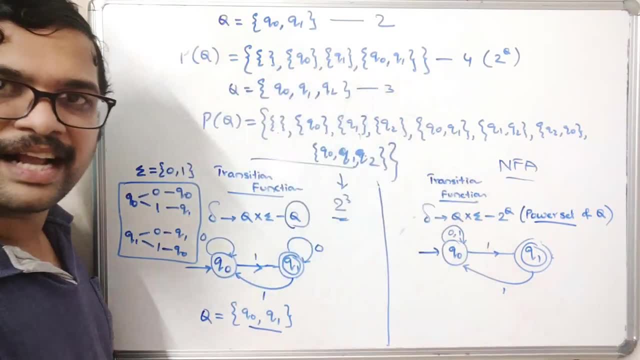 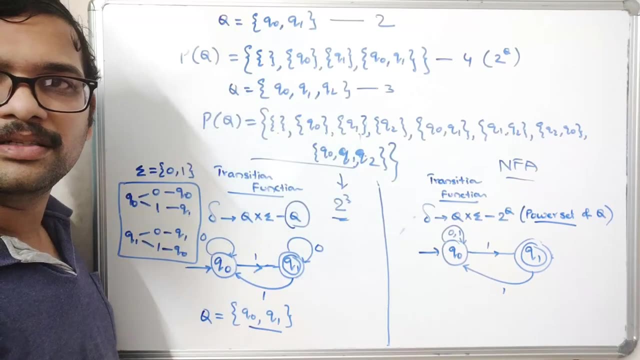 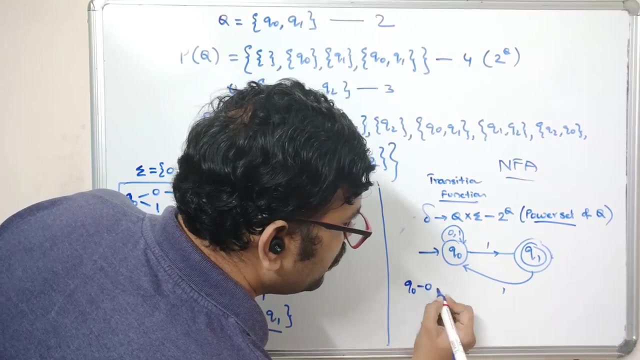 One point is for every state, there need not be a transition for every symbol. And second one for every state with a one input symbol. there can be a multiple states or multiple paths. So here you can observe here: a Q naught on zero, Q naught on zero, It moves to Q naught itself. 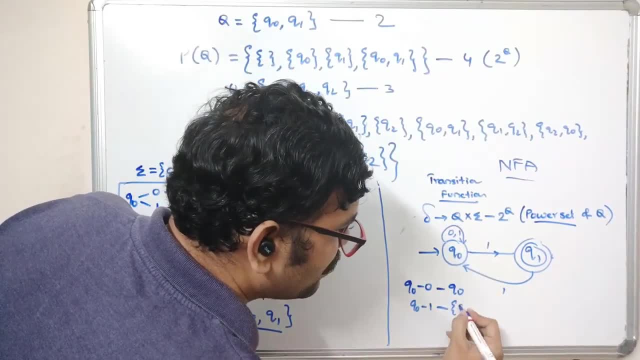 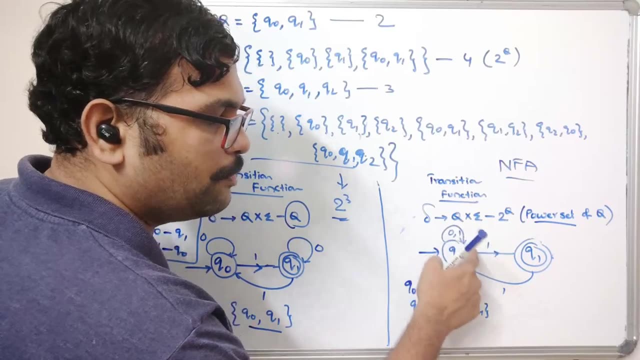 And Q naught on one. It moves to either Q naught or a Q1. Either Q naught or Q1. So here you can have two states for one input symbol. So that cannot be accepted here. That cannot be accepted here, Right. 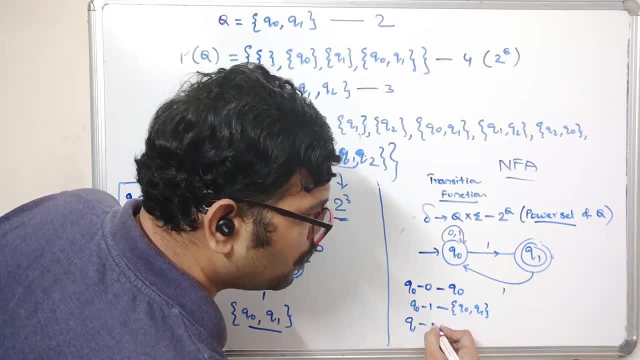 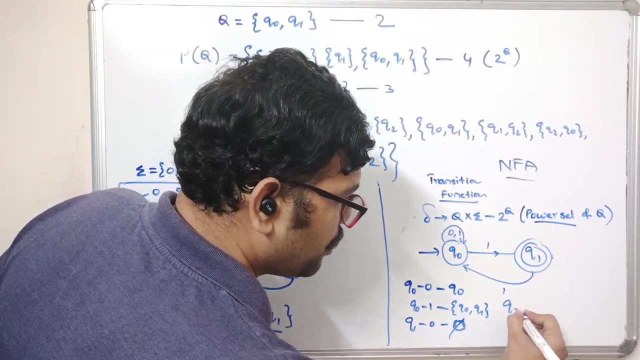 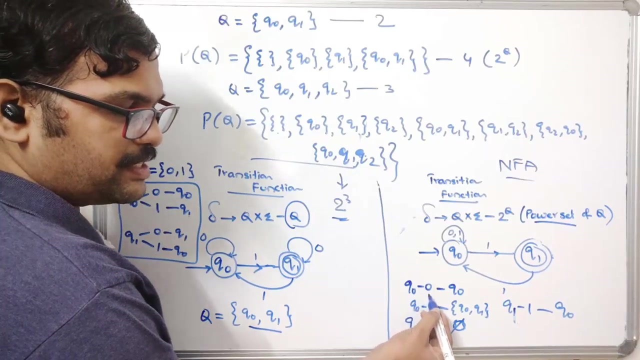 And similarly Q1 on zero. There is no state, So it will be then empty, Right. So or simply we can use a five. Next, Sorry, Q1 on one which goes to Q. naught, You can see for every input symbol, for every transition. 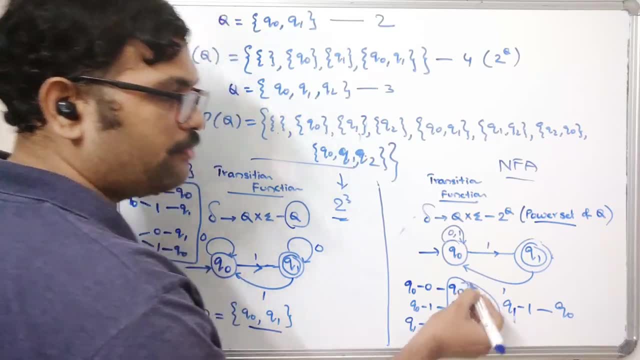 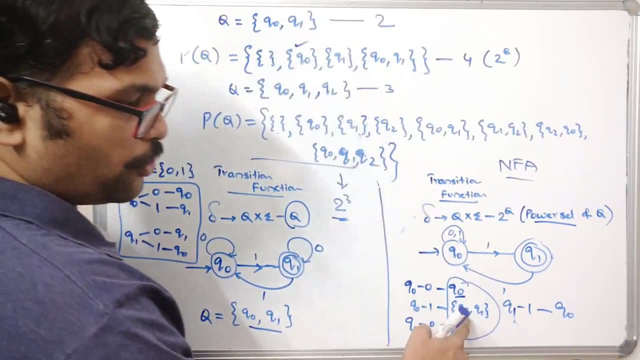 The result will be from the power set, Right From the power set of Q, From the power set of Q. So you can observe here Q naught available in this power set. Yes, Q naught Q1.. Q naught Q1.. 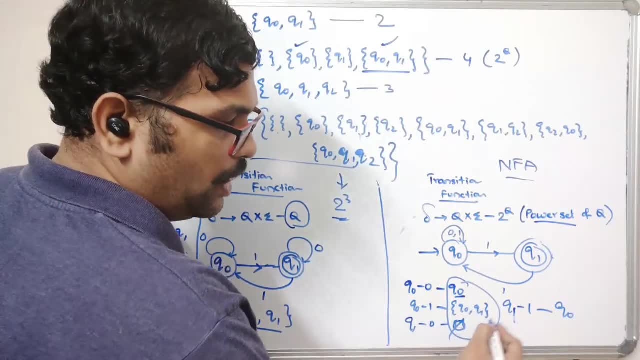 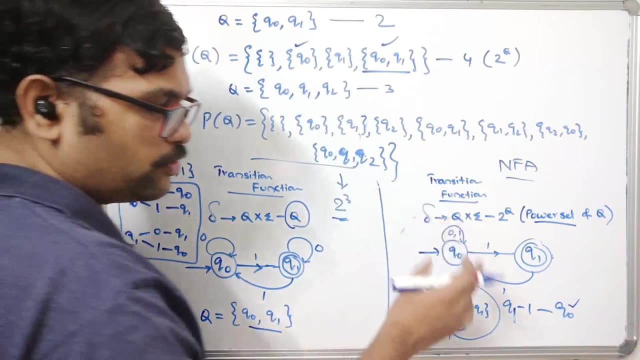 So one element in the power set of Q And next Q naught. So Q naught is one power set in Q, Right? So hope you understood this one. So if you apply any input symbol for one state, it will move with the only one state. 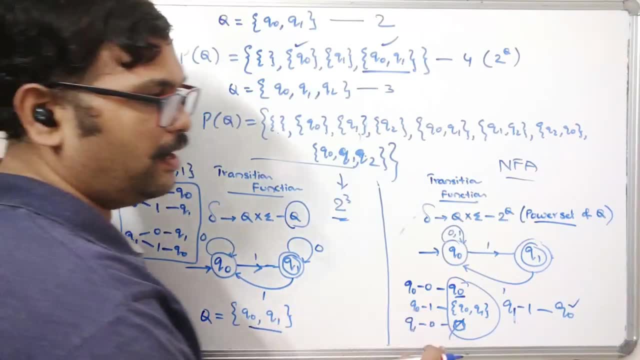 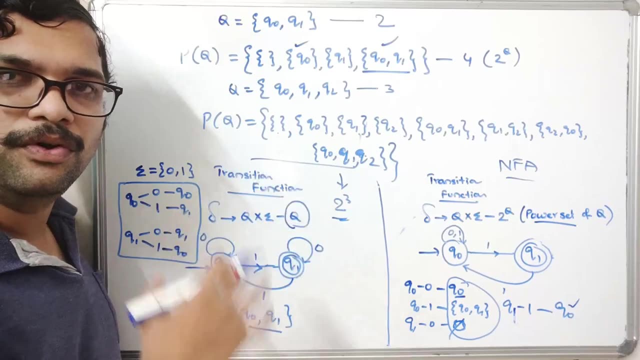 So that will be a subset of Q, Right. And here we will get the resultant state. from the subset of 2, power Q. That means power set of Q. From the power set of Q, we will get the resultant state, The next state, Right. 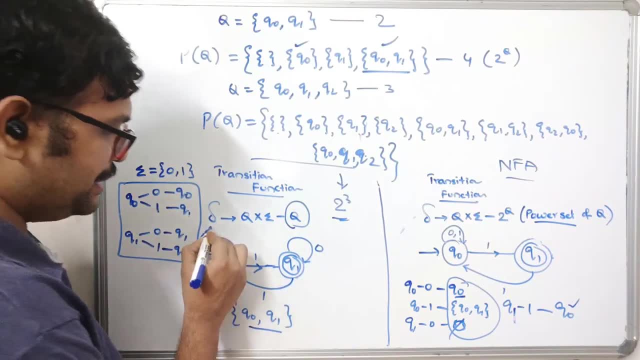 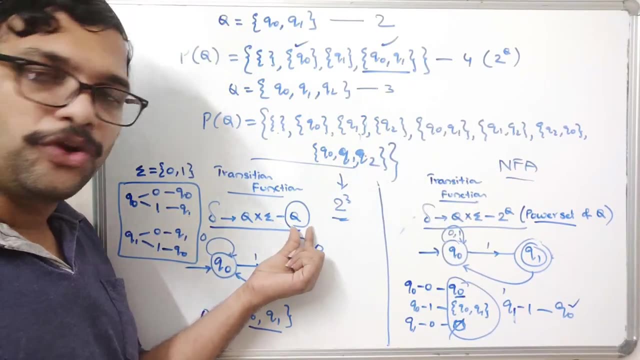 So this is the difference between NFA and DFA. So this is the only difference, is transition function, The transition function. So the resultant will be from the Q Subset of Q, And here the resultant will be the subset of power set of Q. 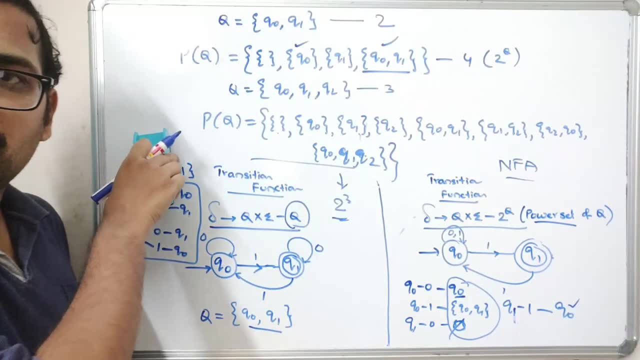 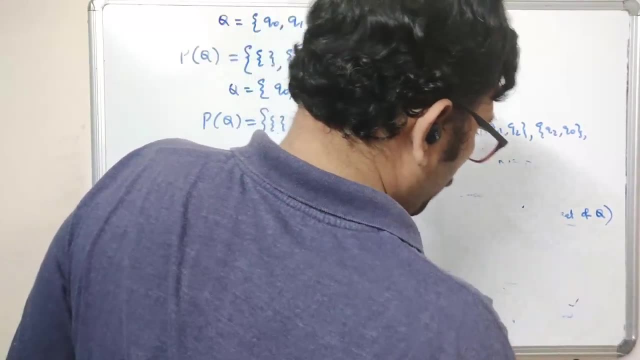 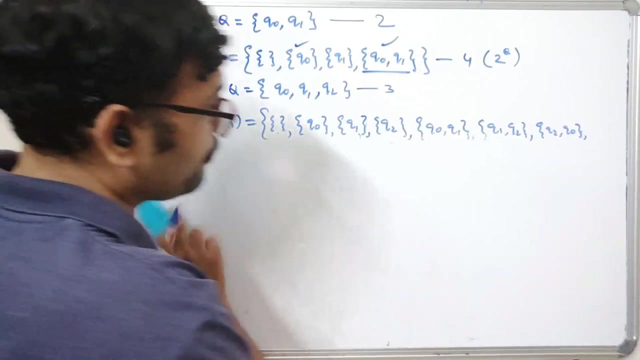 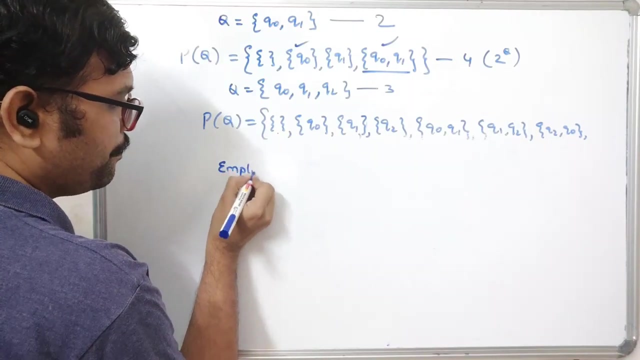 So this is the procedure to calculate the power set. So hope you understood this one: DFA and NFA Right. So hope you understood the basic differences. Okay, Multiple paths and unique transitions. So here the empty transition. 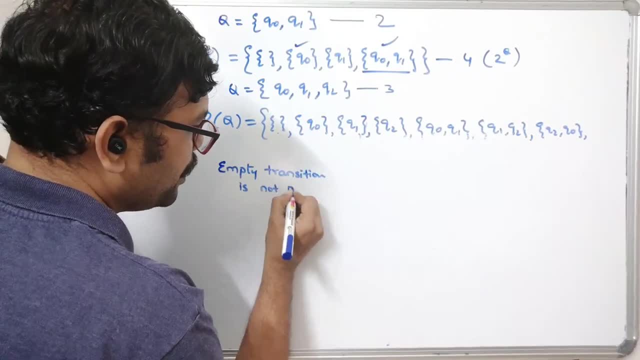 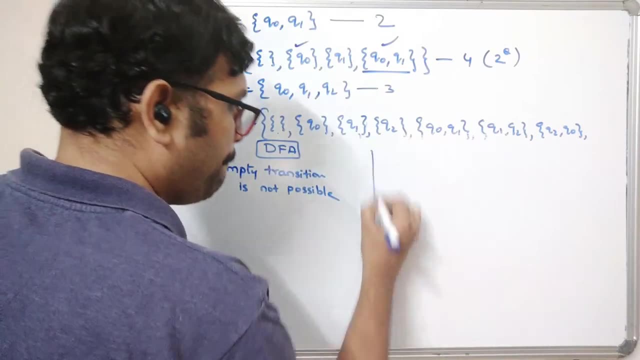 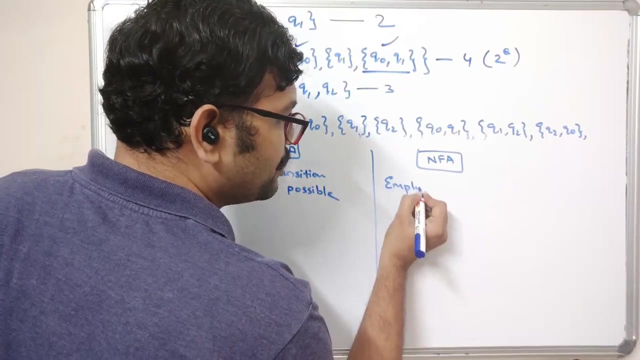 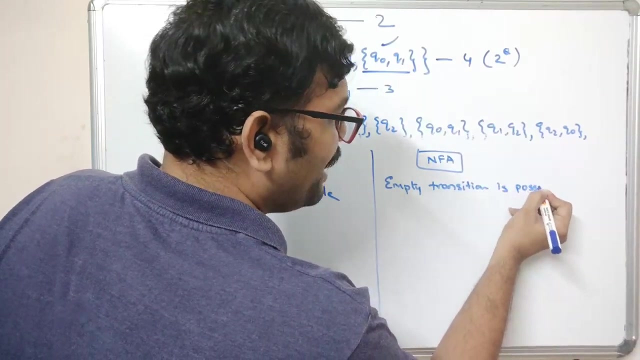 Is not possible. Is not possible. So this is a DFA, Right, This is a DFA And this is a NFA. So here, empty transition, Empty transition is possible, So we can have the empty transition. So in the further sessions we will see about this- empty transitions. 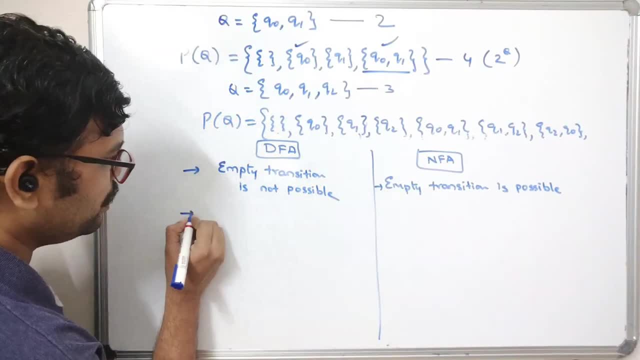 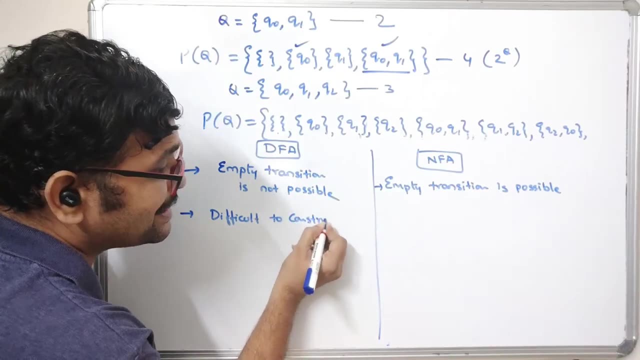 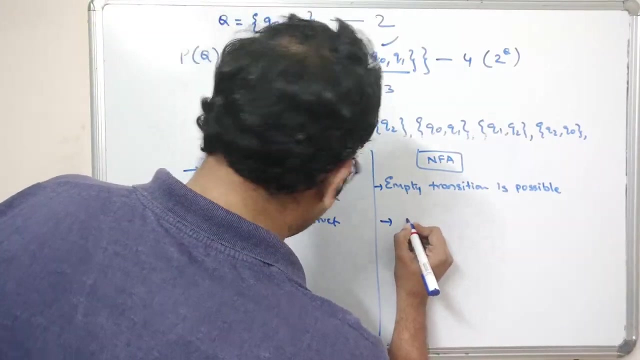 And this is one point And the next one: It is somewhat difficult to construct. Difficult to construct Because for every state there should be one transition with respect to the input symbol, But here it is not required, So construction is very easy. 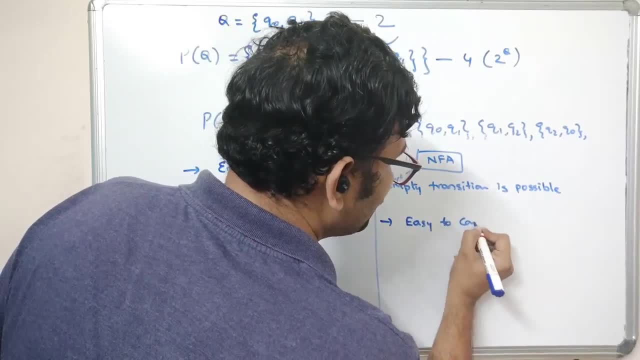 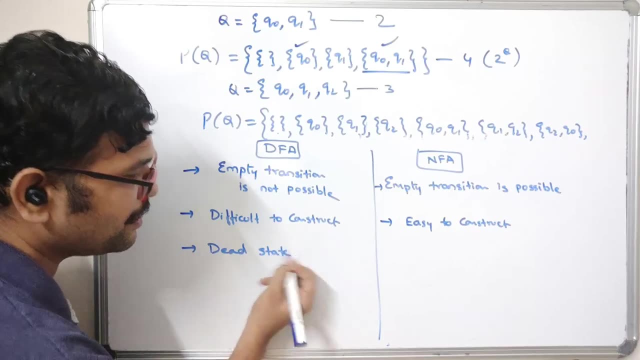 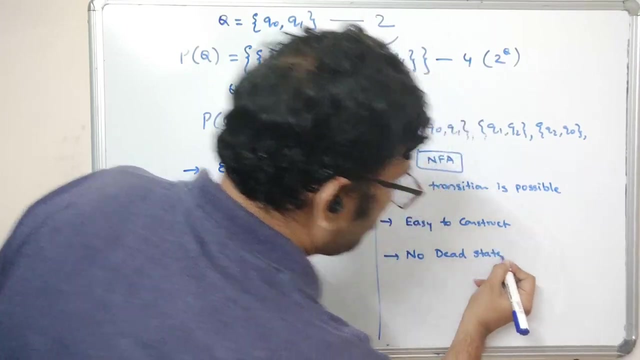 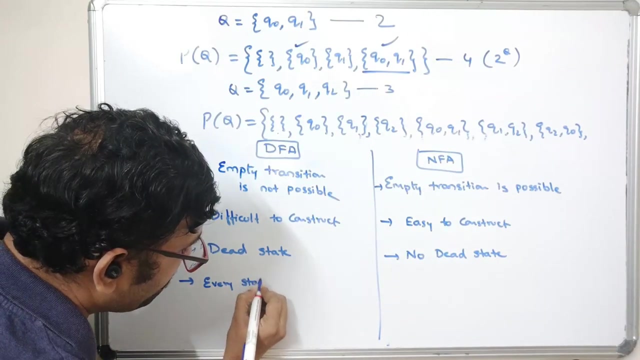 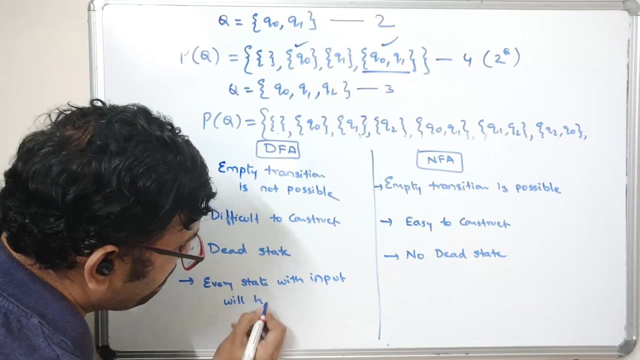 So easy to construct And here we can have the dead state, So dead state is included. So here we are not having any dead state, No dead state, Right, And every state with input will have transition. Okay, Okay. 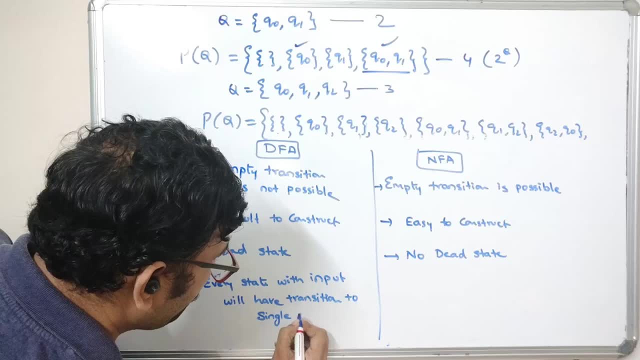 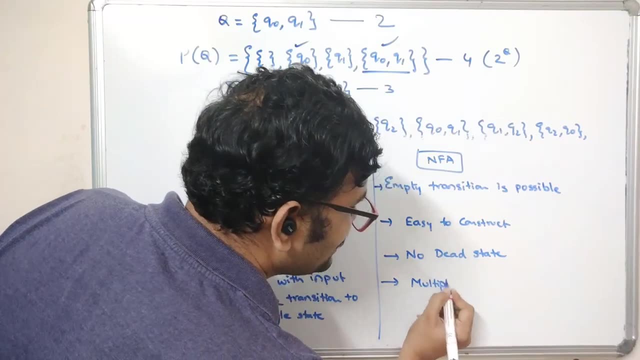 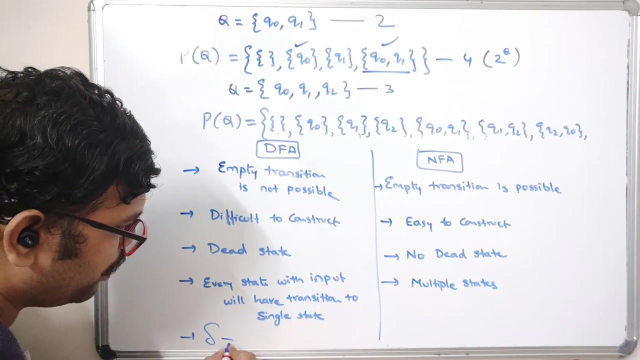 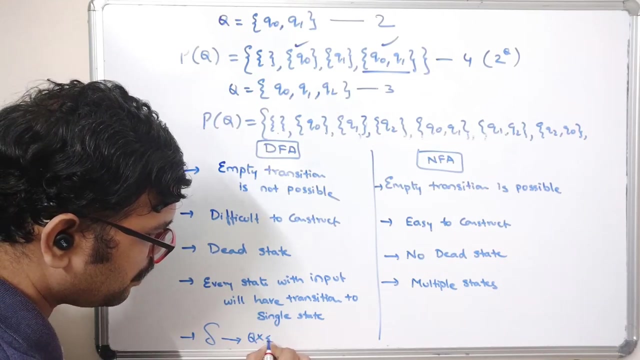 To a single state. Single state, Single state, Right, But here multiple states. So one transition can have a multiple states And a common thing which we have discussed so far, Though, is equal to. That means transition function is equal to Q cross product with a sigma. 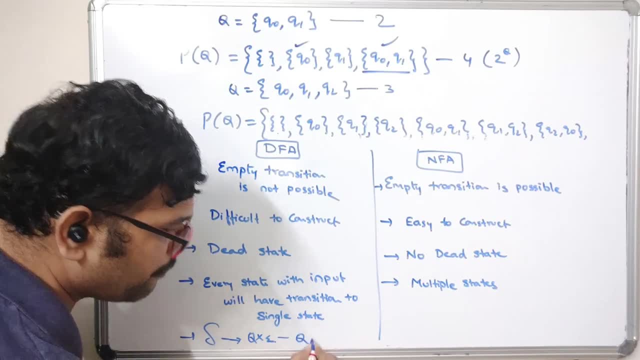 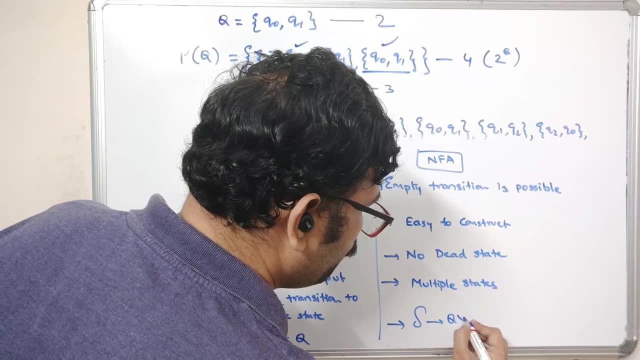 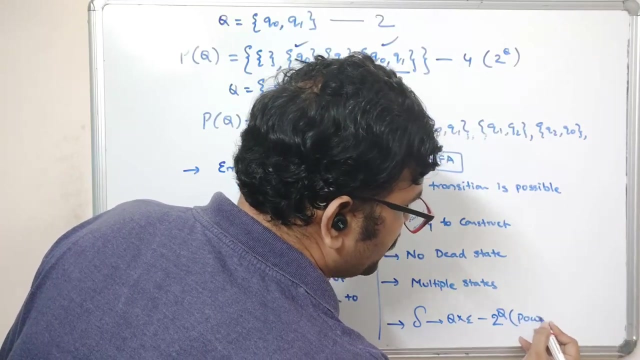 Will give the resultant state from the subset of Q, And here the transition functions. So that means a cross product with a Q, with a sigma, Will give the subset of 2 power: Q. That is a power set. That is a power set. 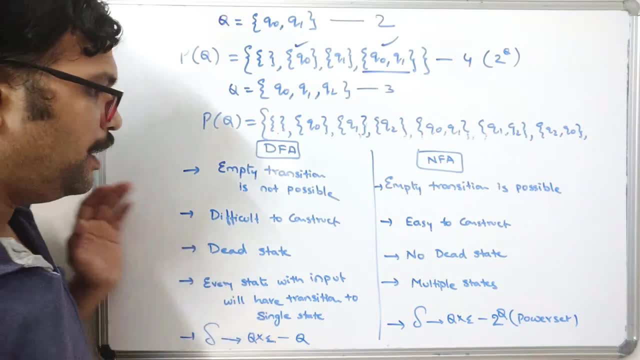 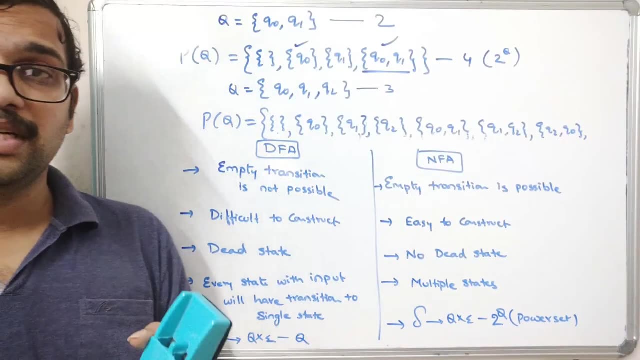 Okay, So power set Right. So these are the some sort of differences between the DFA and NFA. Hope you understood this one, And if you are having any doubts regarding this one, Feel free to post your doubts in the comment section. 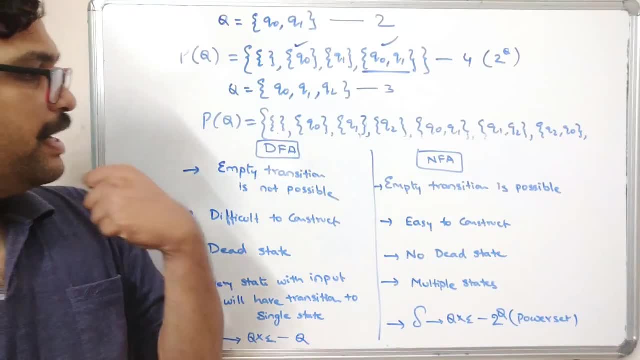 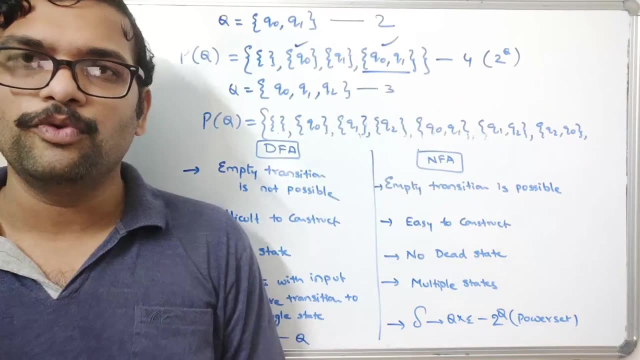 Definitely. I will try to clarify all your doubts And in the further sessions we will go with the DFA constructions and the NFA construction. So first we will see the DFA construction And then we will move on to the NFA construction, Right?